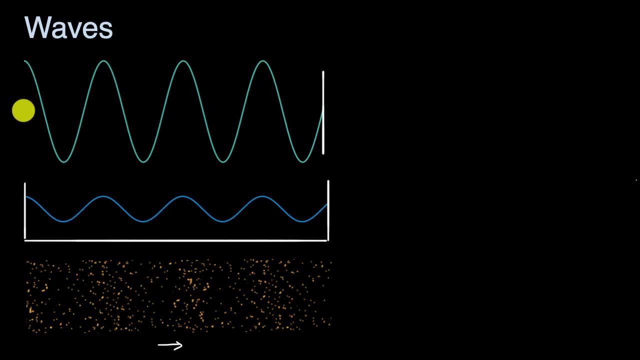 how much are we getting disturbed from what we would call the equilibrium? You could view that as maybe the middle state right over there. Well, if we're getting disturbed that much, we could call that the amplitude. That's how much we are going above or below that equilibrium. 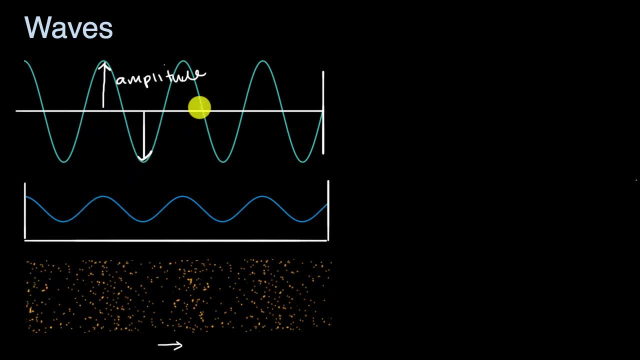 This would be the amplitude as well. We could think about how far is it from the same points on the wave. So if we go from one peak to another peak, well we could call that the wavelength, And you could just do it from any one point on the wave. 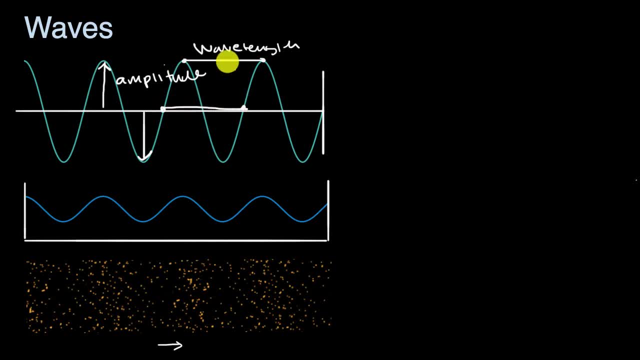 that's just like it on the wave again, So that would be the same wavelength as our original wavelength. right over there You might hear the term frequency of a wave, And one way to think about that is if you were to just observe our original rope. 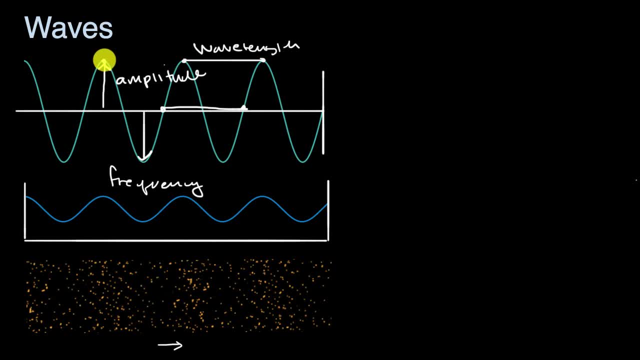 and if you were to say how many times does it go all the way up, all the way down and then back up, So it completes a full cycle? How many times can it do that in a second? If it does that five times in a second, 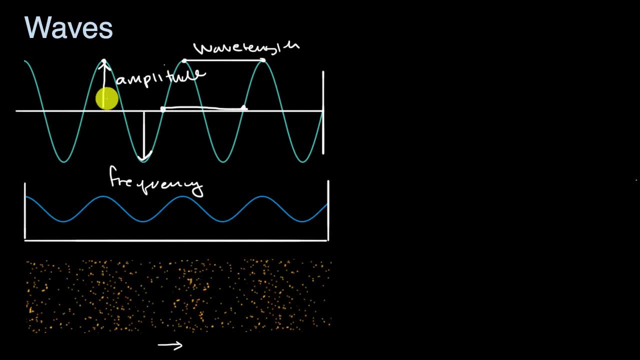 then someone might say it has a frequency of five cycles per second. Now, everything that we have just talked about, these are called mechanical waves. It's a special category, probably the ones that you will see most often. Now. mechanical waves need a medium to travel through. 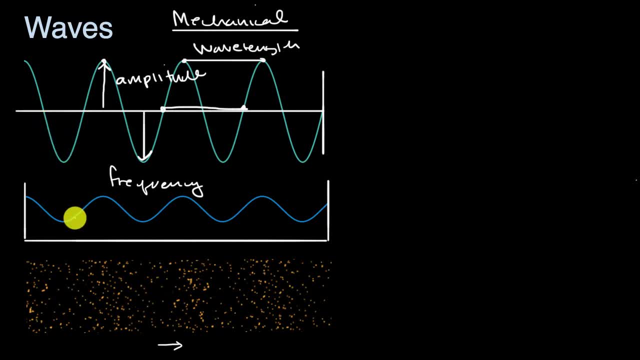 In the rope example, the medium was the rope. The water example it's the water. In the sound example, the medium is the air. Now there are things that can be described as waves that don't need a medium In particular, and this is kind of mind-boggling. 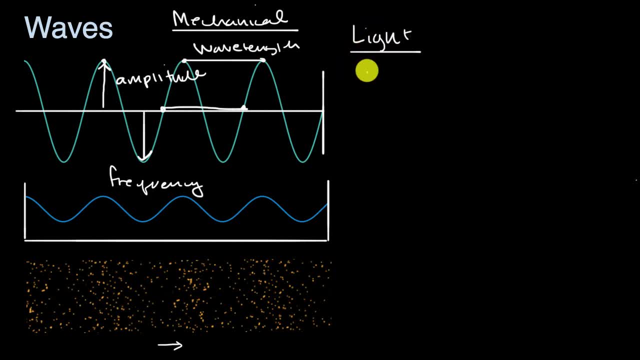 is that light can be considered a wave. If we think about the different frequencies of light, our brain perceives that as different colors. And if we think about the amplitude of light, our brain perceives that as the intensity of light, how bright it is. 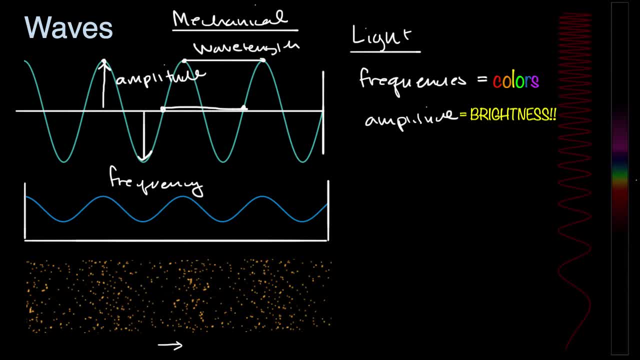 And even more mind-blowing. visible light are just certain frequencies. visible light are just certain frequencies of what we would call electromagnetic waves. There's actually higher frequencies of electromagnetic waves that they have all sorts of applications. You might've heard of ultraviolet light.